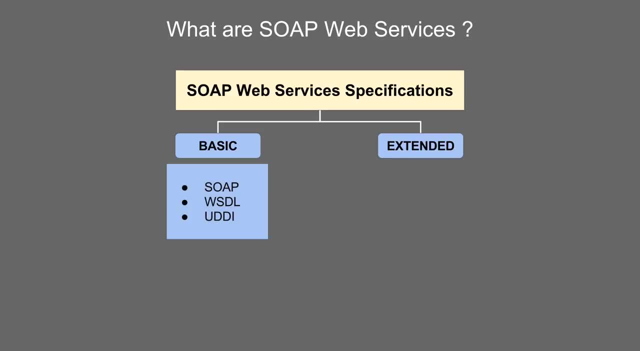 A basic set and it includes SOAP, WSDL and UDDI. So any web service that follows these three specifications can be called as a SOAP web service. And we have already seen about WSDL, which is web services description language, and UDDI in our last session. So, in case you, 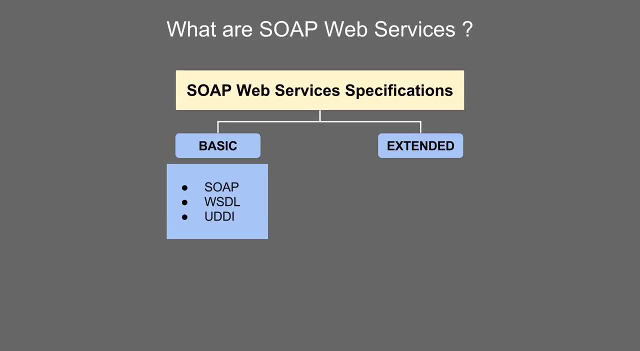 have not seen that session. you can go back and see that session first and then come to this particular tutorial. There is SOAP, which is which we will look into this session more deeply. There are some extended set of guidelines as well, and they include security and other things, And whenever 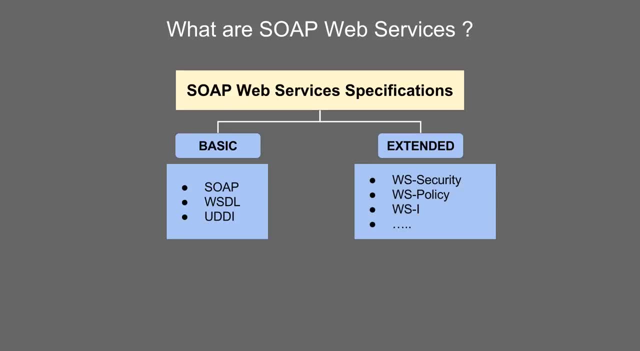 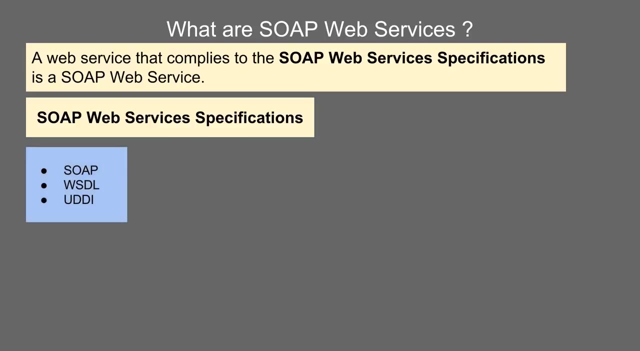 we create web services for enterprise, we follow these guidelines as well, But in this session we will focus on the basic specifications. So we have already learned that any web services that follows the SOAP Web services specifications can be called as a SOAP web service. and these guidelines. 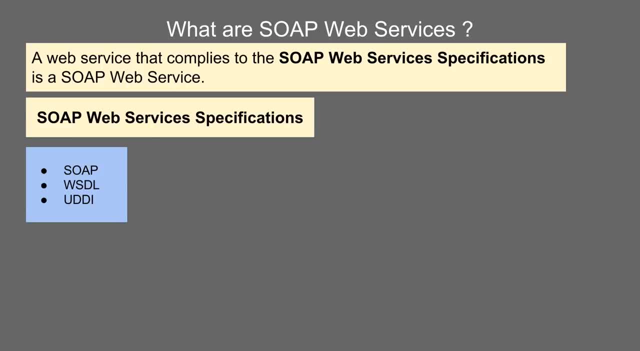 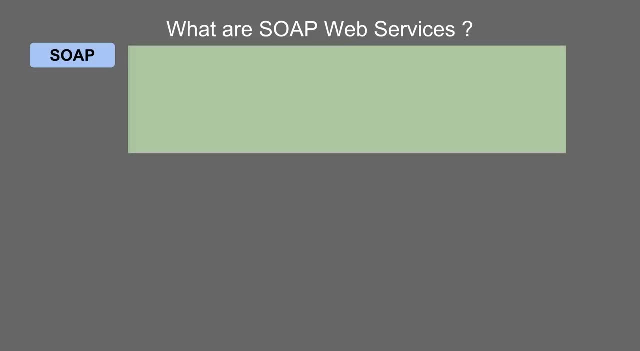 are laid down by a central body, W3C, and there are three basic rules that a SOAP web service has to comply to to actually become a SOAP web service. So let us see what SOAP means. So SOAP is a protocol and it stands for simple object access protocol. Now this is the expansion. 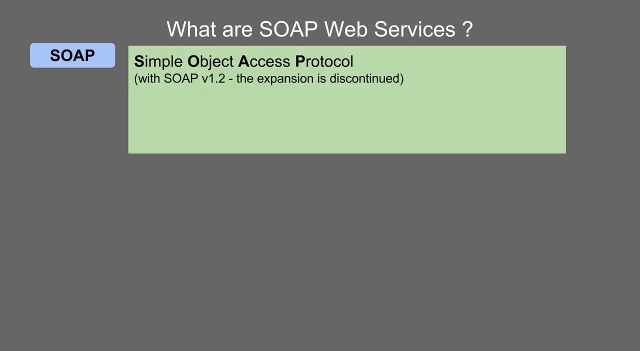 which was used until SOAP version 1.1, but with SOAP 1.2, this expansion has been discontinued, but we are still stuck with the acronym. So it basically is a set of rules and definitions on how two applications will talk to each other over the Internet. 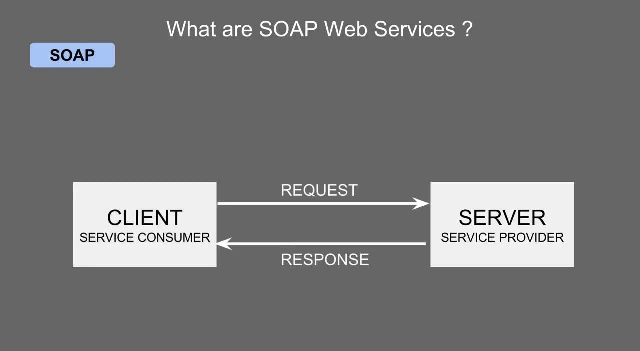 So let us understand this. We know the client server concepts and we know that there has to be a service provider and a service consumer, and they talk to each other with the help of web services. So SOAP protocol says that all the exchange of data or message or information between 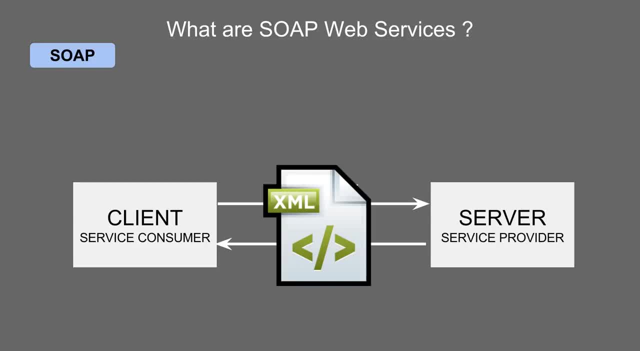 these two application has to be in a format, and that format has to be a common format And in case of SOAP it has to be XML. So all the information and message exchange has to occur over a common format, and the common format that SOAP uses is XML, And it also. 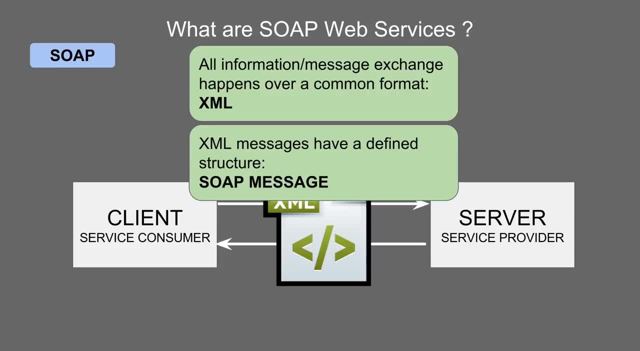 says that it cannot be a very simple XML document. The XML message Has to be a SOAP message, And what we mean by SOAP message is the message should consist of some particular structure, and the structure is made up of an envelope, a header and a. 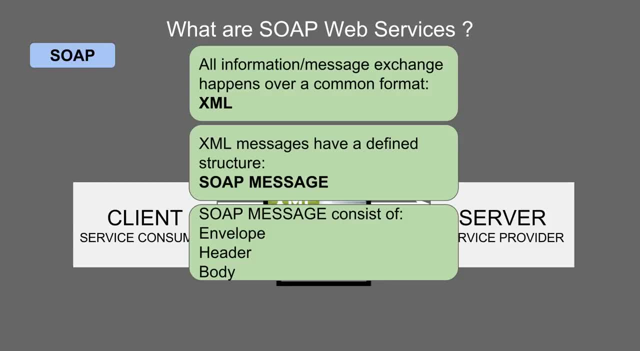 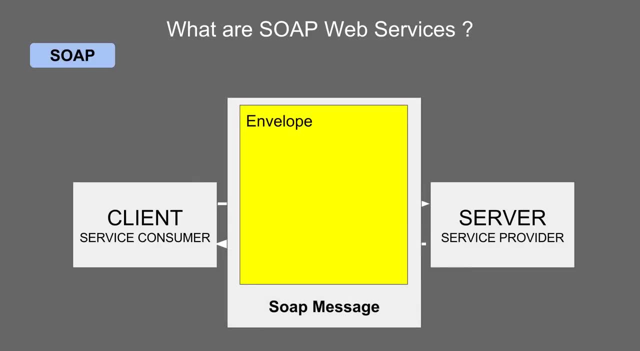 body. So let us look into this: What exactly the SOAP message consists of. So the SOAP message consists of an envelope, which is the root element, and inside envelope we can have a header. Header is optional and it gives us information about that. 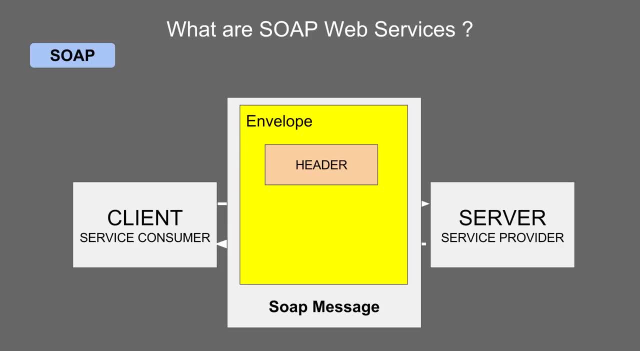 The complex types, and it can have authentication parameters as well. And then we have a body. So let us see: envelope is the very basic, root element of a SOAP message, and it contains other elements like header and body, And header is the element that provides information about the message. 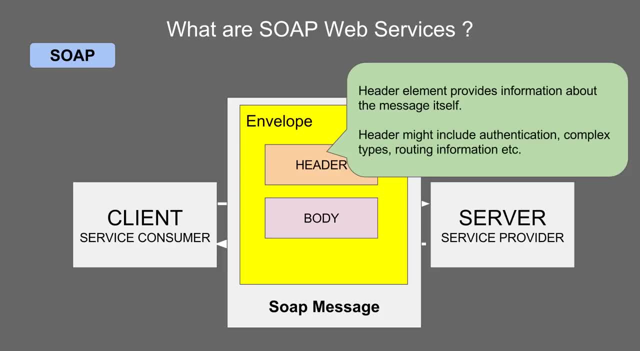 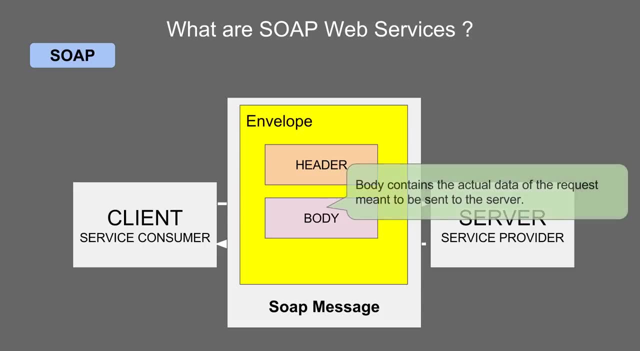 So the actual request is not inside the header, but header can include authentication and complex types and other similar information about the SOAP message, And then we have body, which contains our actual request. So all the parameters that you want to send as a request will be inside the body. 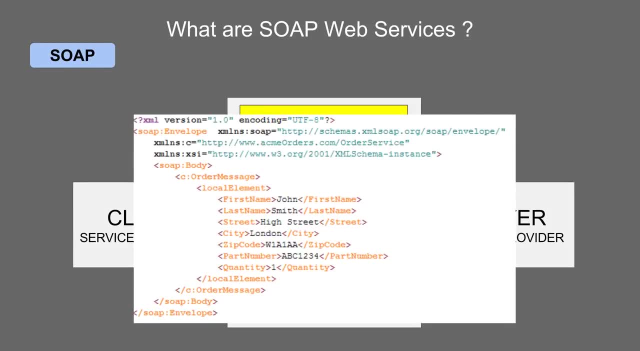 So let us look at this example of a SOAP message. You can see there is the envelope, which is the root element, and we do not have a header, because header is optional. but if you want to give some username, password and some complex, 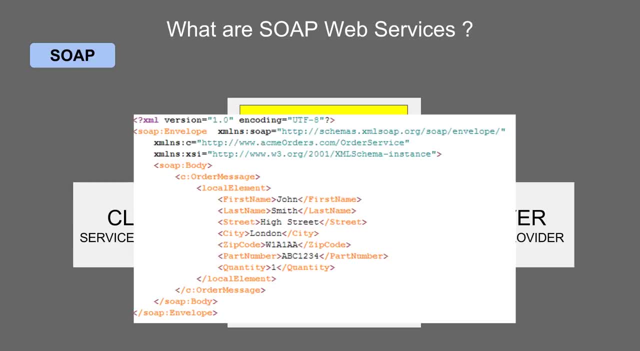 type information That will go inside the header, and then we have a body which has the actual parameters of the request, like first name, last name and so on. So this is what a SOAP message looks like, and any SOAP web services will comply to these. 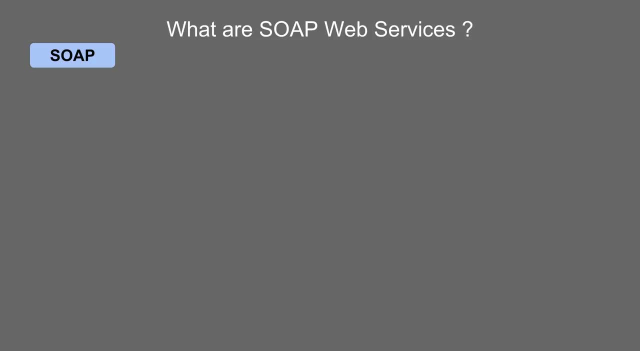 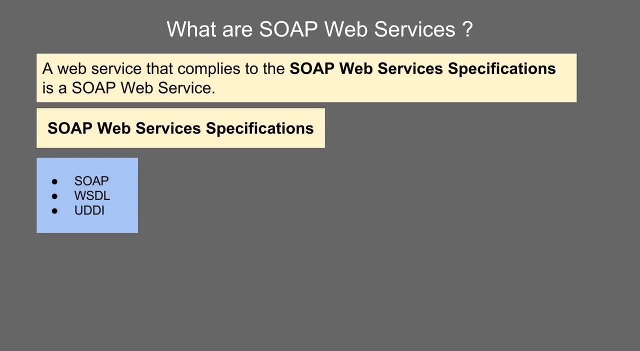 standards of SOAP message. So now let us summarize. We have learned what SOAP web services are. SOAP web services are web services that comply SOAP web services specifications, and these specifications are some guidelines which are laid by a central body, which is W3C, and the basic set of specification.